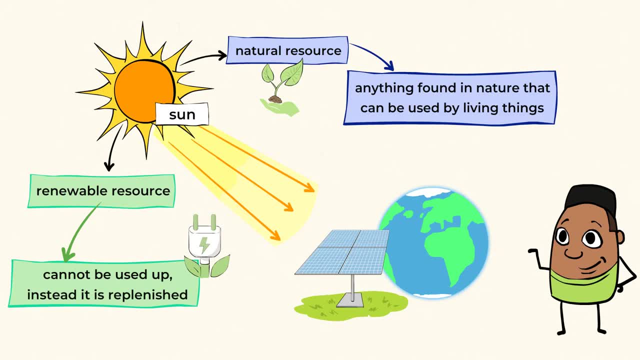 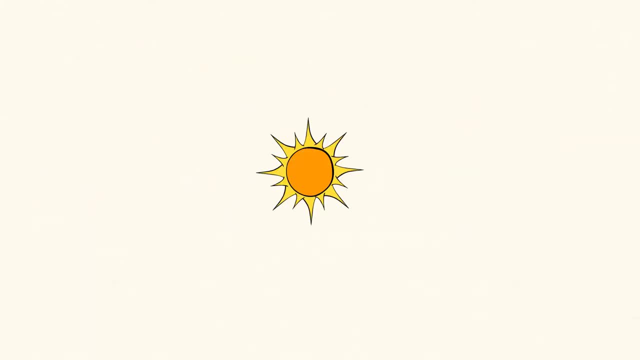 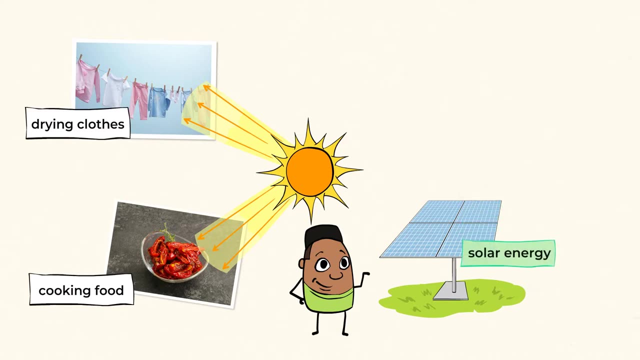 So that makes the sun's energy a renewable resource. We call the energy that we get from the sun solar energy In its simplest form. we use the energy from the sun for things like drying clothes and sometimes cooking food. Humans have also figured out how to use energy from the sun to create electricity. 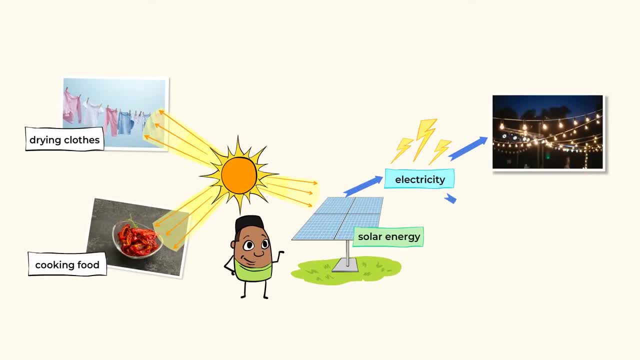 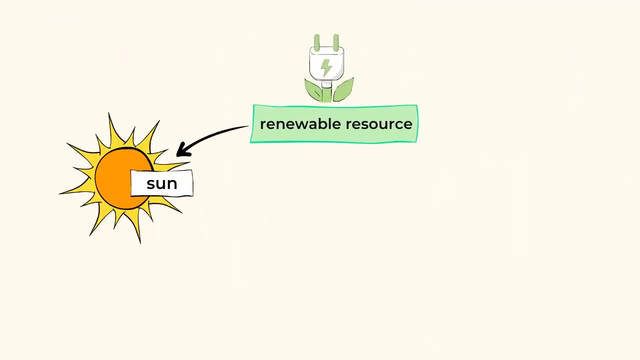 to power everything from string lights in the garden to entire buildings. But the sun is not the only renewable source of energy. Wind and water are also renewable resources, and they can both be used to generate energy. First, let's look at how wind is used to generate energy. 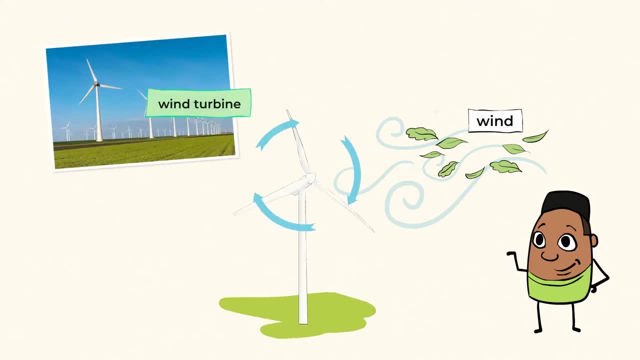 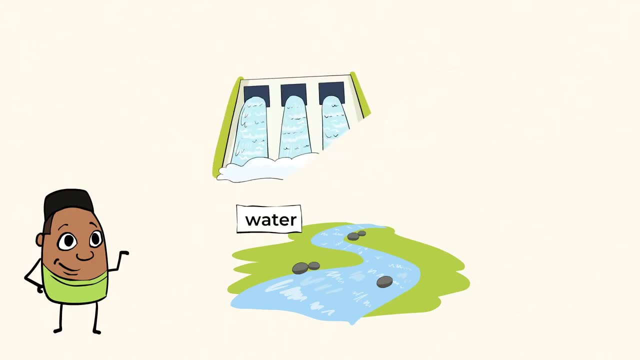 Well, the blades of the wind turbines are turned by the power of the wind, which then creates electricity, And we can use water in a similar way to generate power. Hydropower is power generated by the wind. Water is generated from moving water. 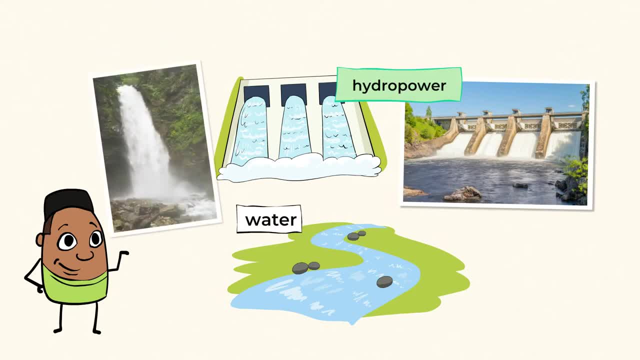 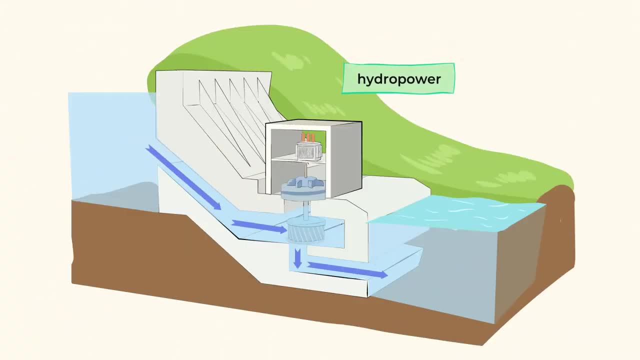 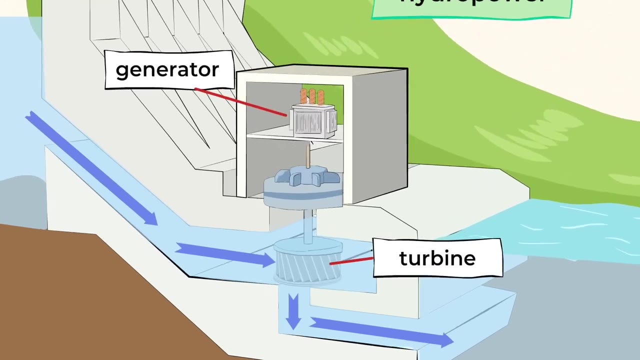 Just think about how powerful a waterfall can be, or the sea waves. Hydropower uses the power of water to create electricity. Water is pushed through wheels called turbines. A generator is connected to the turbines. The spinning turbines cause the generator to spin, which you guessed it. 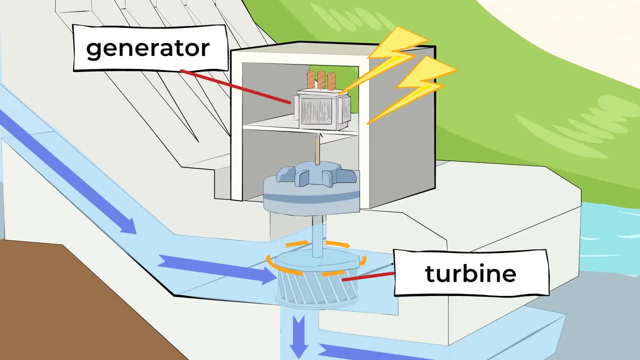 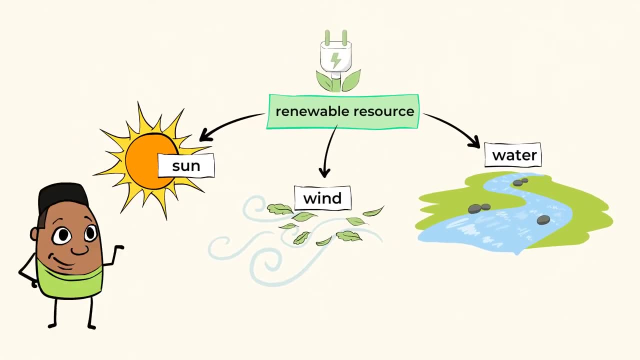 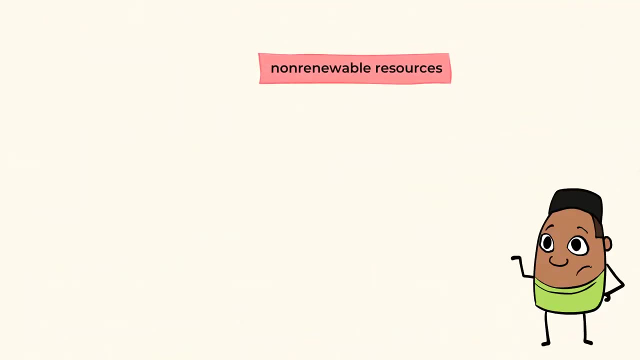 converts the energy from the flowing water into electricity. Those three renewable resources are pretty amazing. But that makes me wonder: are all forms of energy renewable? Well, no, There are types of energy that are non-renewable. Non-renewable resources cannot be replaced when they're used up. 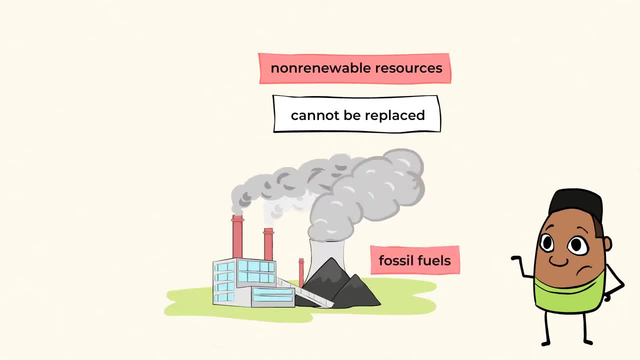 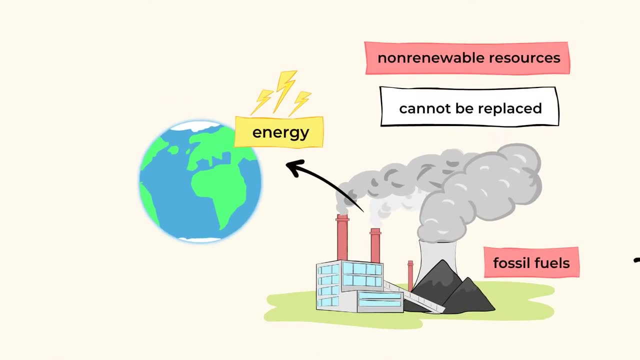 One example of non-renewable energy is fossil fuels. We use fossil fuels every single day and they make up most of the world's energy. So what are fossil fuels? The gas that we put in our cars comes from fossil fuels. 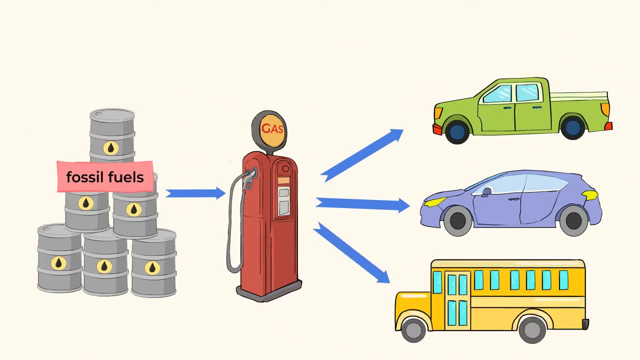 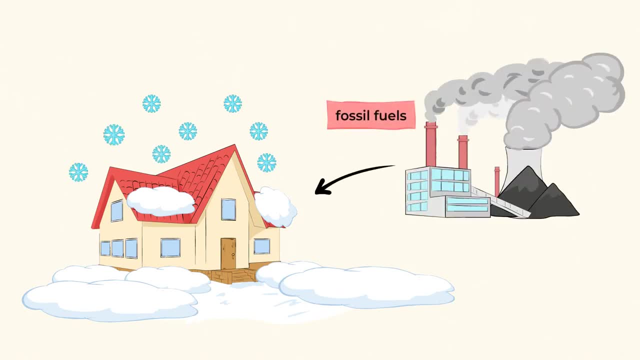 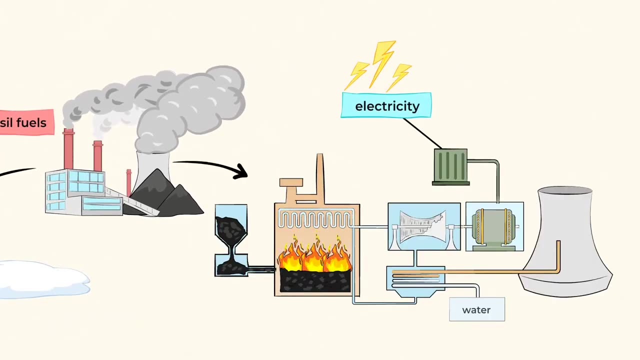 That's right. Almost every car, truck and bus on the road is fueled by gas, And in the winter, fossil fuels are what we mostly use to keep us nice and warm. Many power plants burn fossil fuels to generate electricity. Fossil fuels- they get their name because they're made from prehistoric plants and animals. 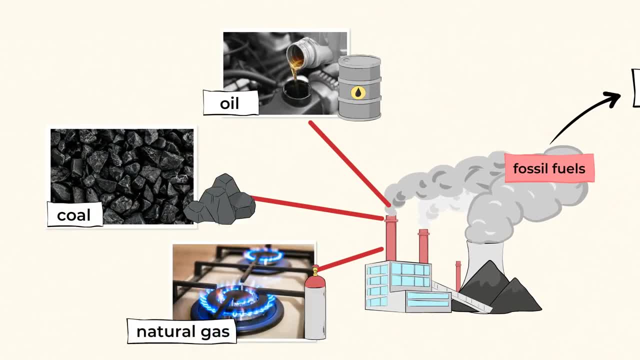 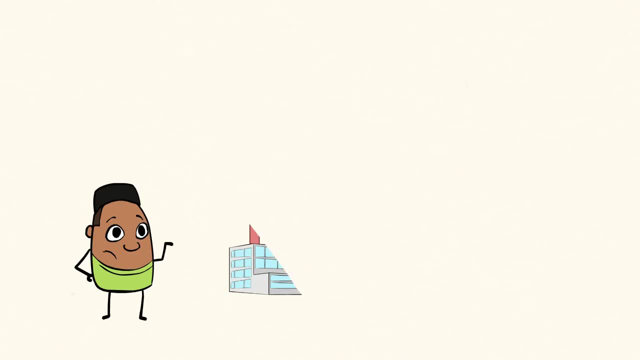 Yeah, that's right. Oil, Oil, coal and natural gas are all fossil fuels, and they make up most of the sources of energy that we humans use Now. fossil fuels are very useful, but they're not always the best choice for an energy source. 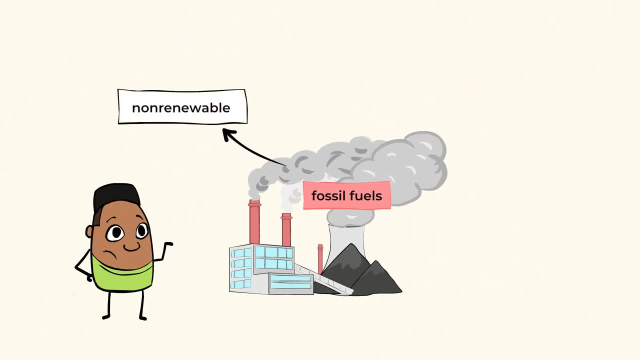 First of all, they're non-renewable, which means we'll run out of them eventually. And, even more importantly, fossil fuels are not good for the environment. When they're burned, they cause pollution which is harmful to the Earth and all the living things on it. 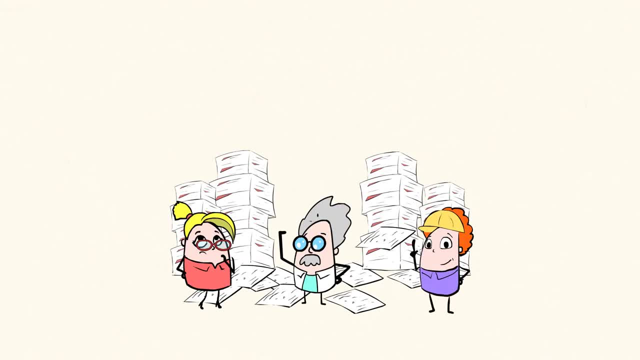 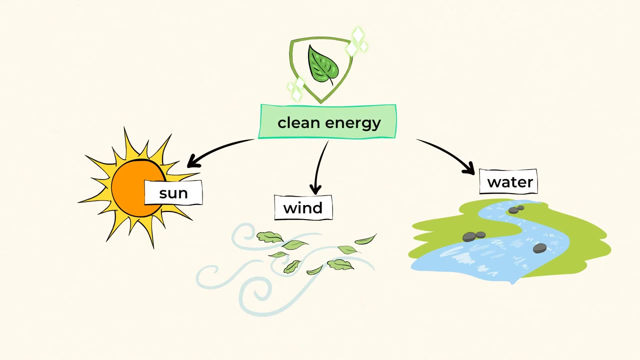 And that's why it's so important to use fossil fuels. It's so important that scientists and engineers keep exploring new ways to generate energy using renewable resources that have less negative effects on the environment. Wind, water and solar energy are all much cleaner energy sources that don't pollute the environment. 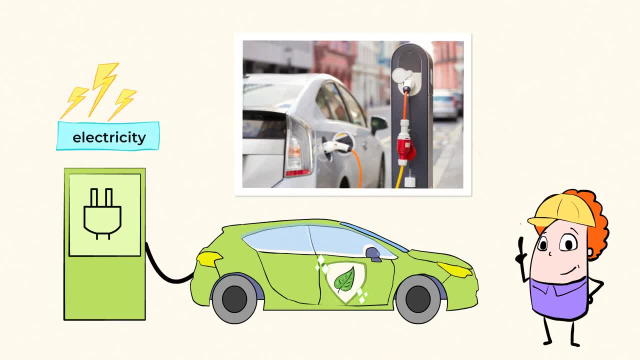 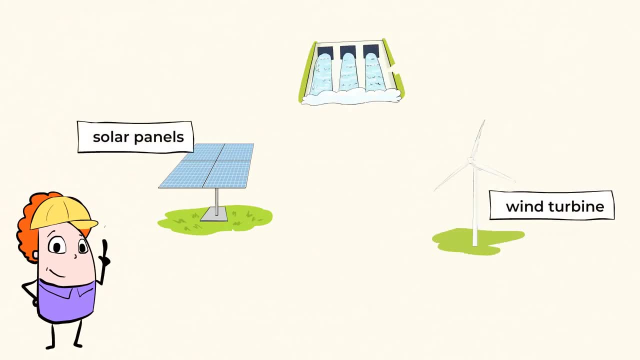 Engineers have already created cars that run on electricity instead of on fossil fuels, And similarly they've developed solar panels, wind turbines and hydropower plants to generate electricity for buildings. And who knows, Maybe one day you'll be the one discovering even more efficient renewable energy sources. 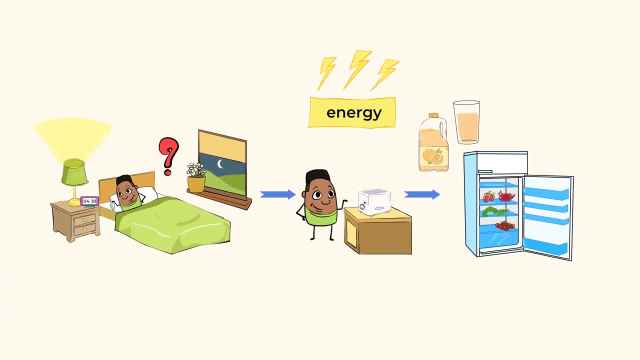 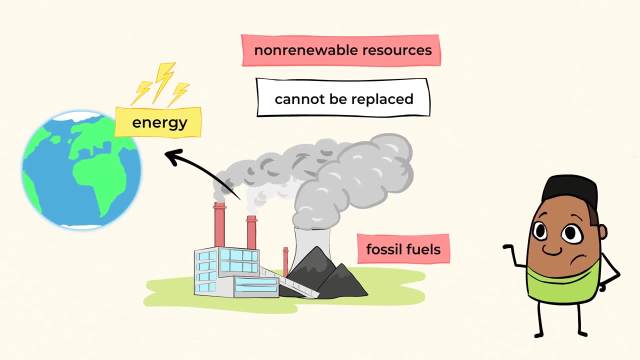 We use energy for so many things in our everyday lives, From the time we wake up until the time we lay down to go to bed at night. Non-renewable energy sources, like fossil fuels, are the most common types of energy we use. 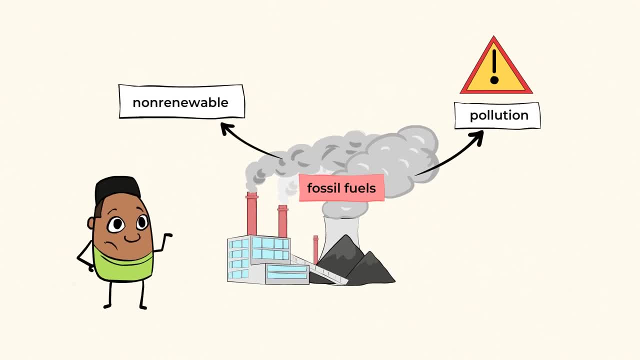 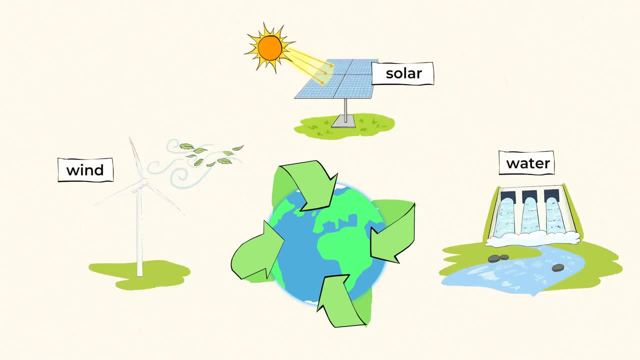 But we'll eventually run out of them And they're not good for our environment. So renewable energy sources like solar, wind and water power are better options for energy because we'll never run out of them and they're not harmful to the environment. 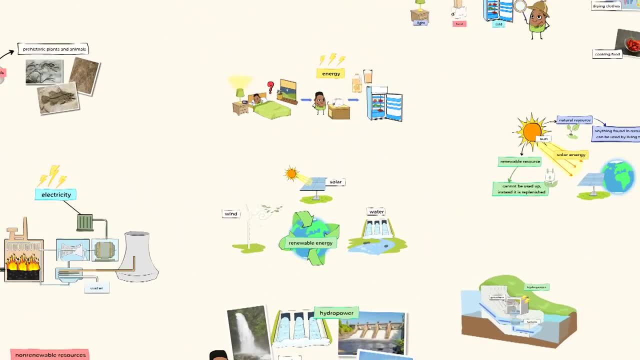 So get inspired and good luck, my mighty scientists, on your path to inventing new techniques and ways to use renewable energy.